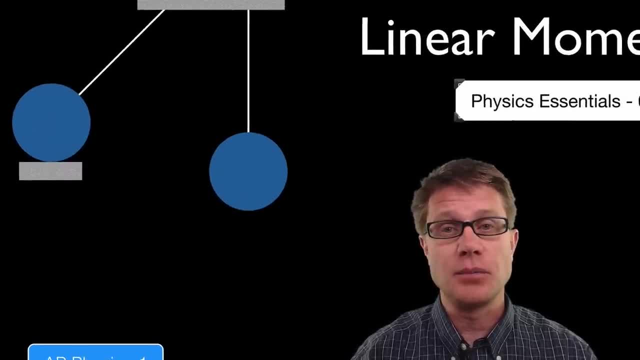 momentum that it has. And I am going to give the blue sphere on the left a little bit of momentum by removing the platform And it bounces off the other sphere and then it comes back again, And so is linear momentum conserved. Yes, It is always conserved in every collision. 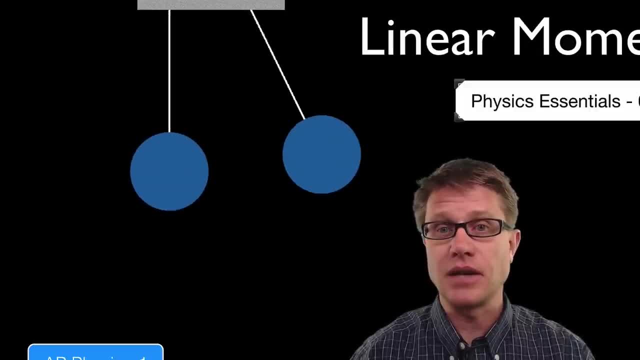 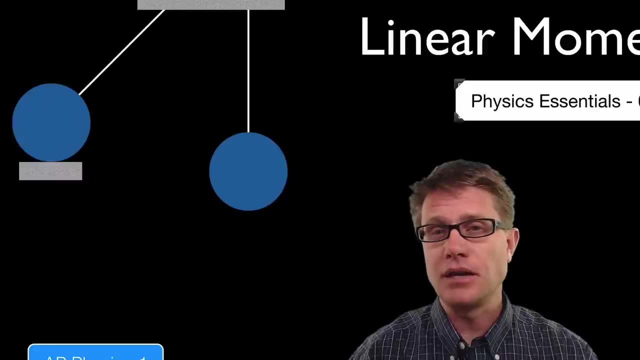 I have momentum on the left side, I am transferring that to the right side And then it is simply coming back again. And this only works if they both have the same exact mass. But what would happen if I made it out of a different material? Let's say I made it out of clay. 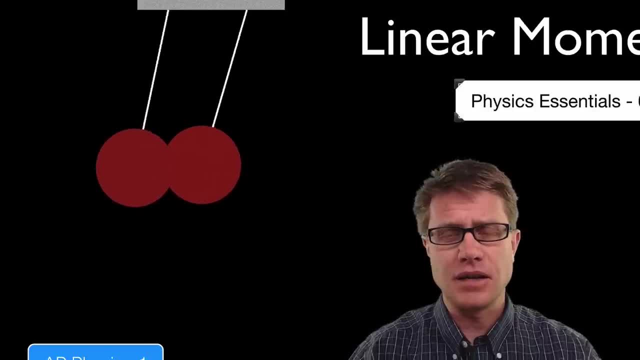 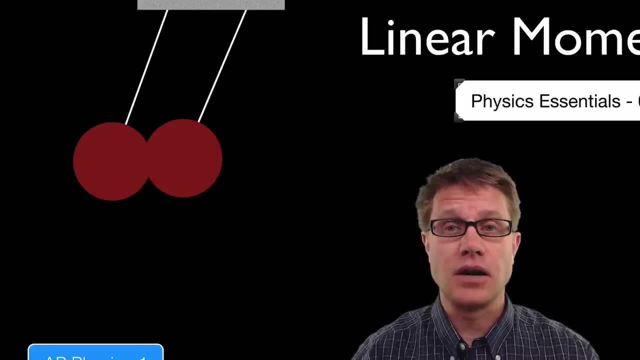 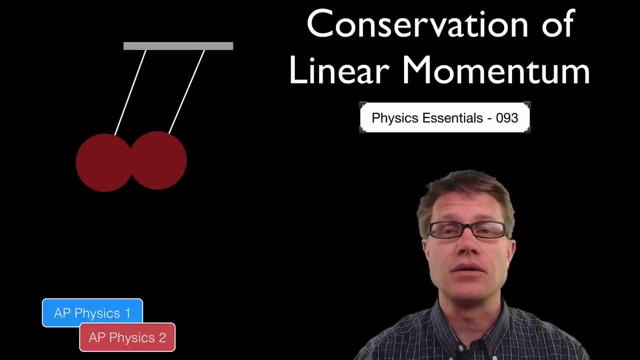 Watch what happens here, Instead of just bouncing off, they come connected to each other, And so what is really lost? We are losing some of that speed. We still conserve our linear momentum, but we lost some of that kinetic energy. And if we lose kinetic energy, we call that an inelastic rather than an elastic collision, And so conservation. 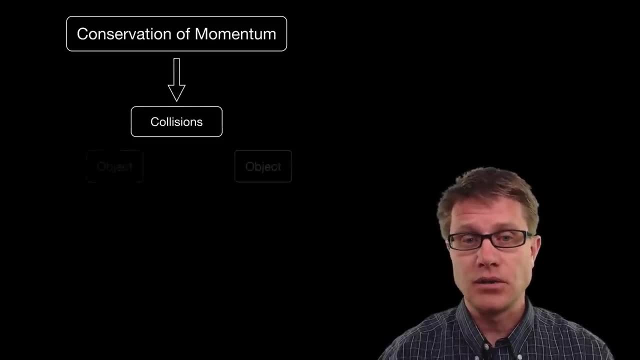 of momentum, remember, is always maintained in any collision. So if I have two objects running into each other, the momentum that we have before the collision equals the momentum that we have after. So let me set up a little elastic collision, like that We are transferring. 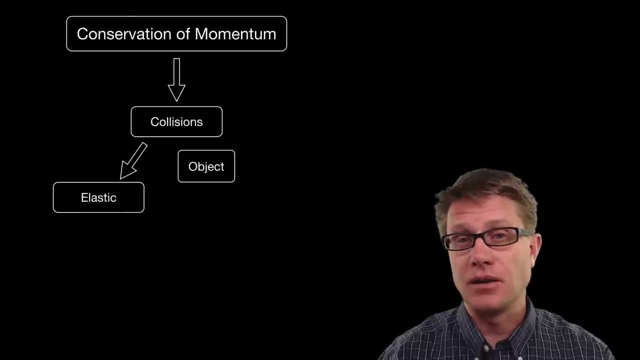 momentum, in this case from one object to another. We would call this an elastic collision. Why is that? Not only have we maintained the linear momentum, but we have also maintained our kinetic energy. We have not lost any of that speed, In other words, the kinetic energy. 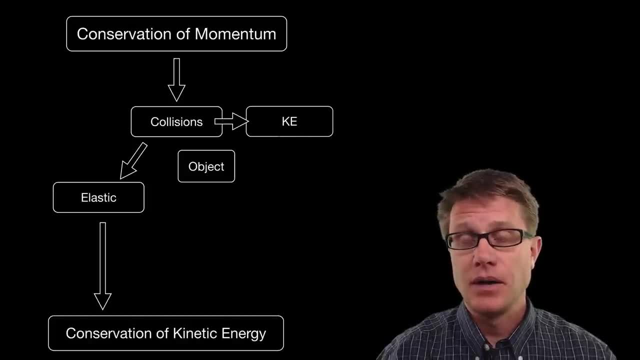 that came into the collision equaled the kinetic energy that came out. Now we could also have another type of collision, called an inelastic collision, And that is when one object hits another object and they lose some of that kinetic energy. Maybe they become connected. 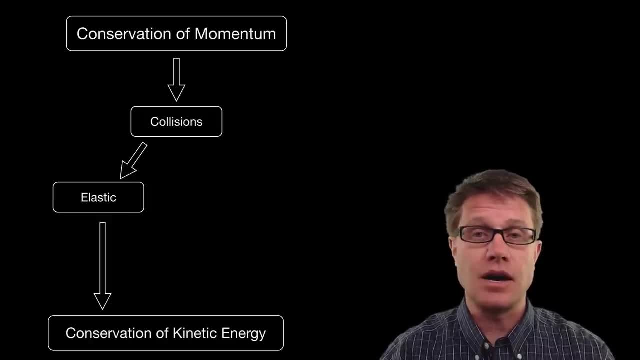 or it could just run into a wall where they both eventually come to a complete stop. So that is a complete stop. We would then call that an inelastic collision. Did we maintain conservation of linear momentum? For sure, We always do in every collision. Did we maintain? 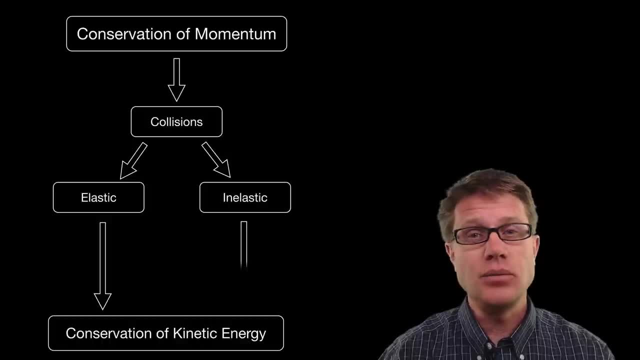 kinetic energy. No, We have lost some of that speed. Did we maintain energy? Is there a conservation of energy? We did. Where did that energy go? It went to the internal energy inside the objects involved in that collision. And so an example of this: if I drop a basketball, 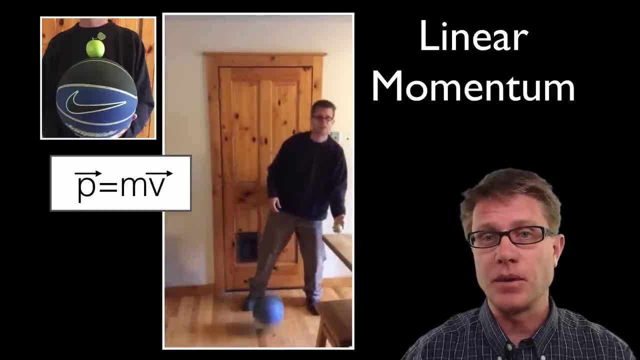 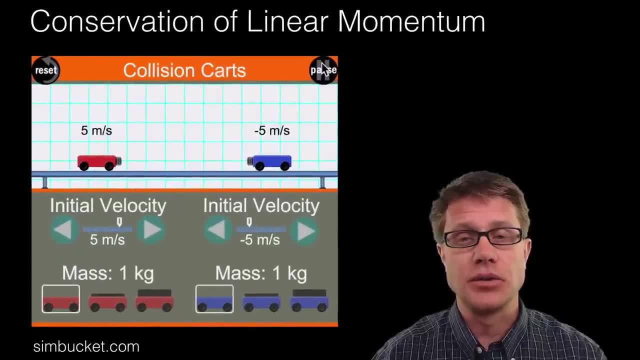 with an apple on the top of it. we are converting some of that momentum forward. We are going to get some from the basketball, which is bigger to the apple. We are increasing its speed. Now the best way to verify this is through experimentation. So we are using a simbucket. 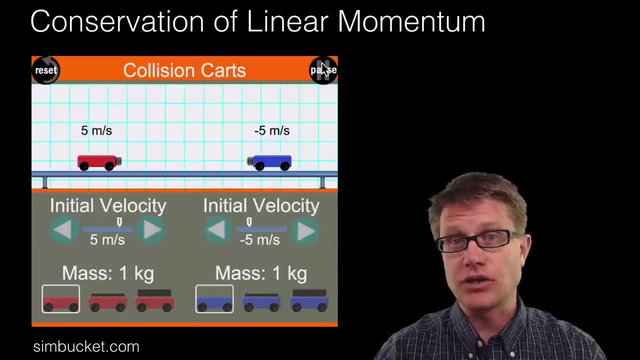 simulation. We have got these carts that are going to collide with one another And it will show us what their velocity is after the collision. And so what we will do is figure out: does the linear momentum maintain, And then does kinetic energy maintain? to figure: 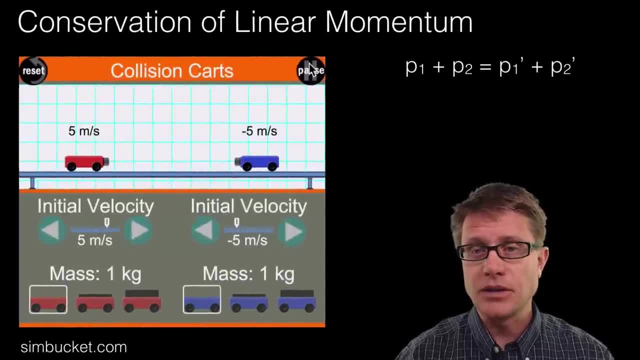 out if it is elastic or inelastic. And so linear momentum, remember, p1 plus p2 equals p1 prime plus p2 prime. And then we are going to use a simbucket simulation to figure out if it is elastic or inelastic. And so linear momentum, remember, p1 plus p2 equals p1 prime. 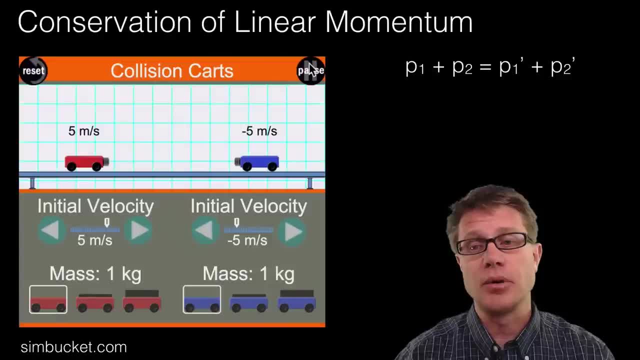 plus p2 prime. In other words, the momentum of those two objects before has to equal the momentum after, And so let me give this collision. You could see in this simulation that both of them have a 1 kilogram mass. to begin with, Initial velocities were 5 meters per second. 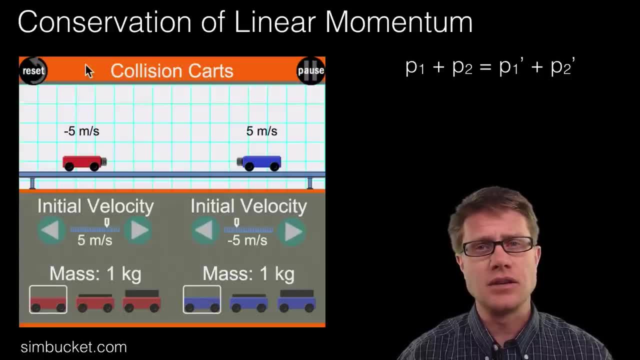 on the left, Negative 5 meters per second on the right, And you can see that those speeds are reversed after the collision. And so if we set up our equation, m1 v1 plus m2 v2 equals m1 v1 prime, that is, after the collision plus m2 v2 prime. So I can just plug that. 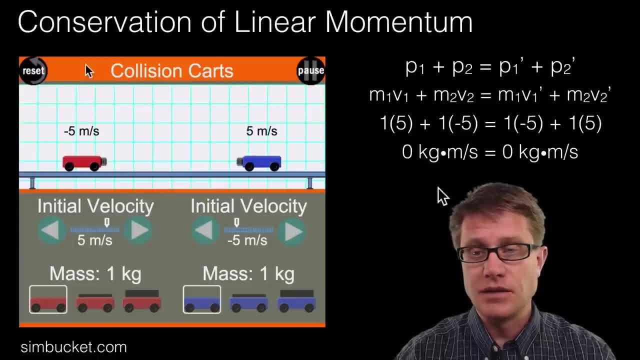 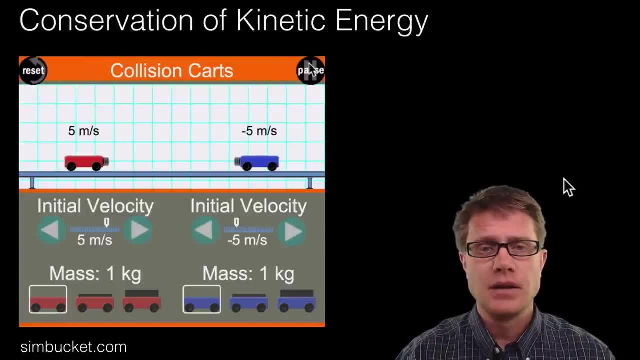 and 0 after Linear momentum is maintained. Now is kinetic energy maintained. in this collision, Kinetic energy before and after is going to be equal. Well, if we do that collision, it looks like the speeds are not changing very much, And so I then have to get to the math. 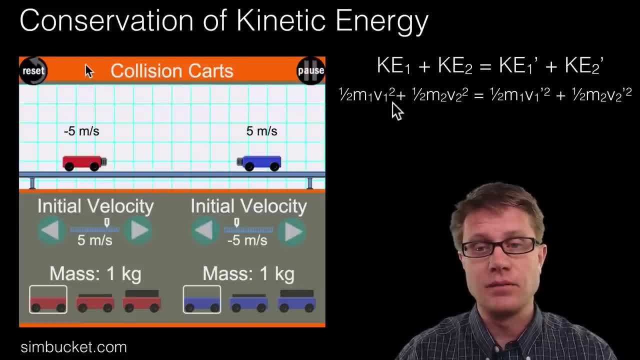 And so I am going to plug in kinetic energy. This looks scary, but again, it is 1 half mv squared plus 1 half mv squared of the objects before the collision and then after the collision. So if I plug in those values, what I find is 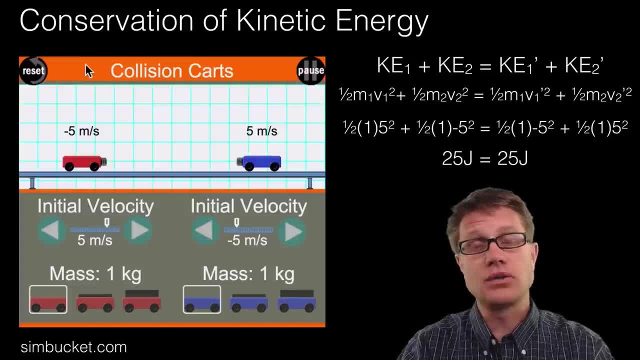 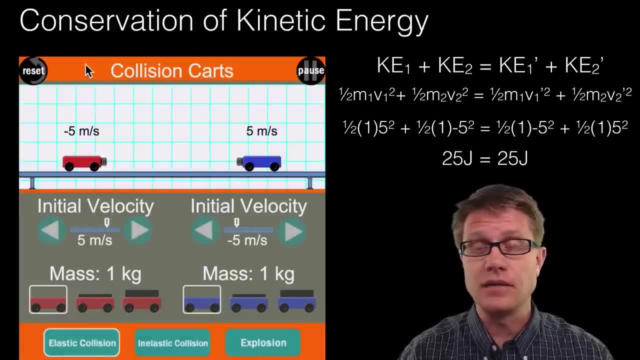 that we had 25 joules of kinetic energy before and 25 joules after, And so is this an elastic or an inelastic collision? It is elastic. We have not lost any of that kinetic energy. Let's try another one Now. the one on the left has 10 meters per second, So it has got. 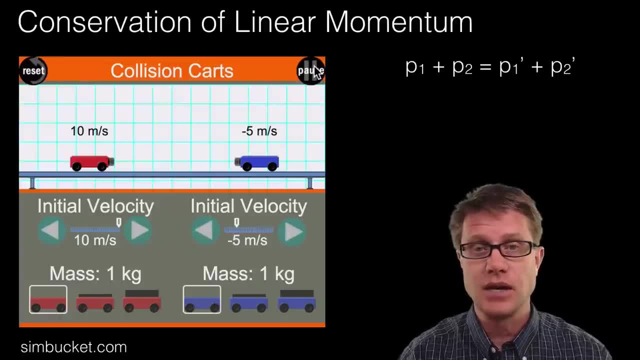 a greater speed than the one on the right. They both are 1 kilogram, So the one on the right has 1 kilogram masses. You could guess as far as what is going to happen when they collide with each other. You can see the speeds are going to be swapped, And so if I were, 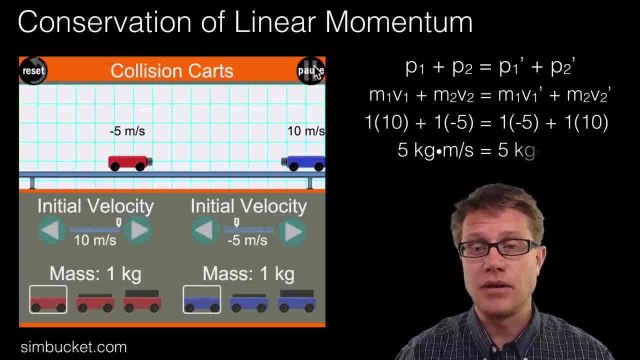 then to plug that into my linear momentum equation, I would find that the momentum we had before is equal to the momentum that we had after. Now it is not 0 anymore. What is it? It is a positive value That indicates that we have a shift, In other words, the overall. 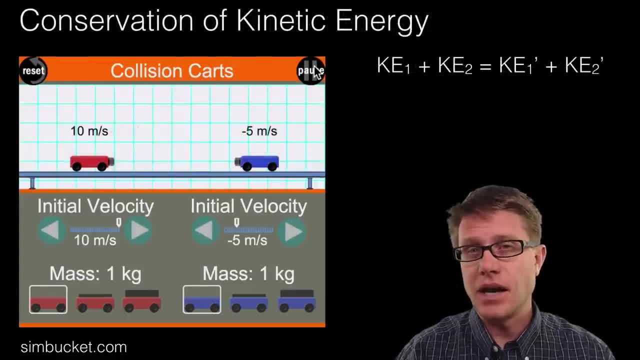 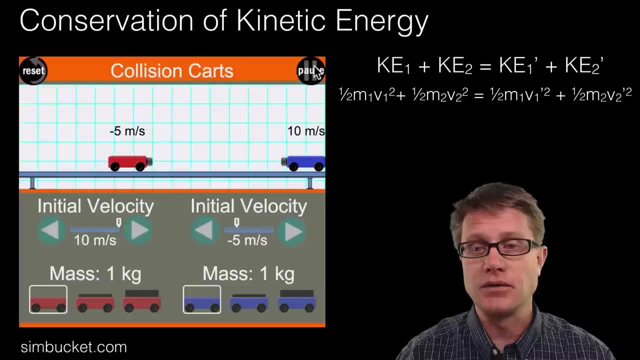 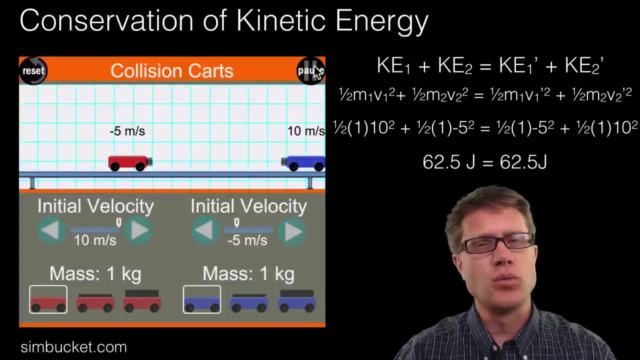 momentum is to the right in this system. Now is kinetic energy maintained. Again, we use that formula: Kinetic energy before, kinetic energy after. If I plug those values in, what I find is that we have 62.5 joules before, 62.5 joules after. Now we have more kinetic. 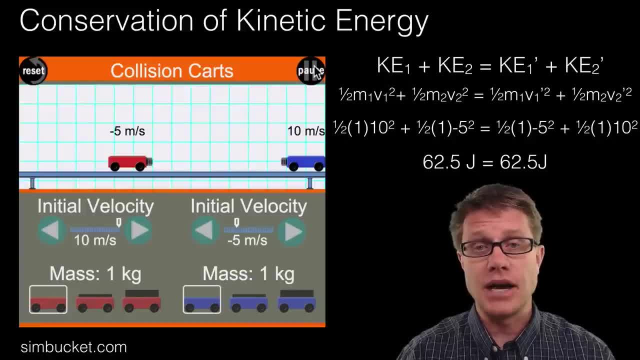 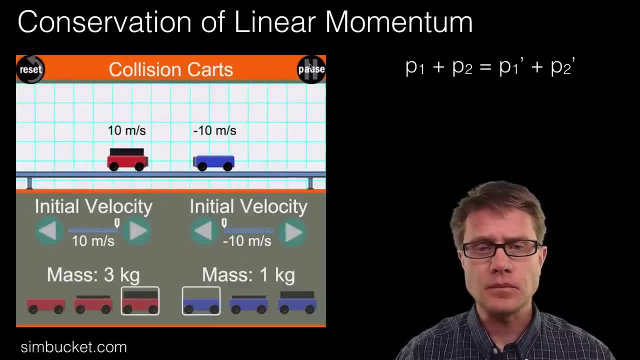 energy because one of those cars is going faster. But is it an elastic collision? For sure, Because we have maintained kinetic energy. Now let's go to a different kind of a collision. Instead of bouncing off of each other, they are becoming connected, And so you know right. 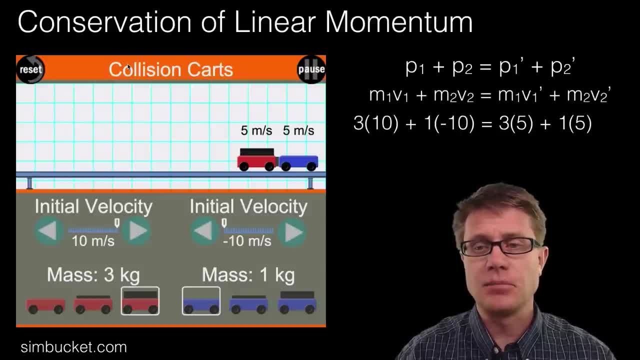 away. this is probably going to be an inelastic collision. This is probably going to be an inelastic collision. If I plug in my linear momentum values, I find that the momentum we had before 20 equals the momentum we have after. Again, it is always going to be maintained. 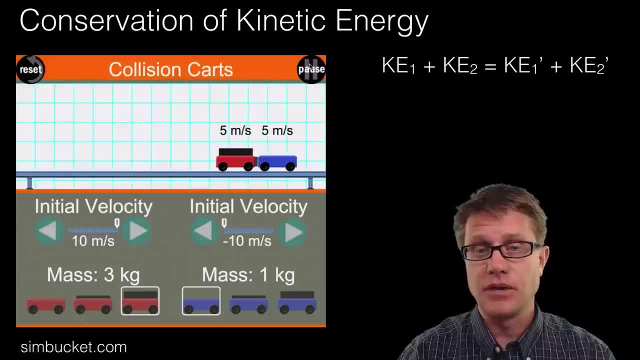 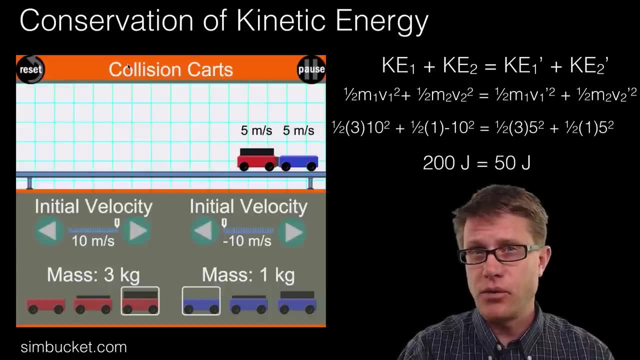 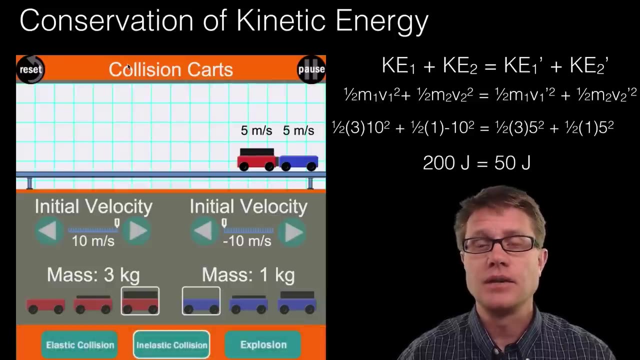 But then if we look at the kinetic energy before and after and we figure out our values, you can see that we have less kinetic energy after. If I plug in those values- 200 joules before, 50 joules after, And so we have lost 150 joules of energy. What does that indicate? 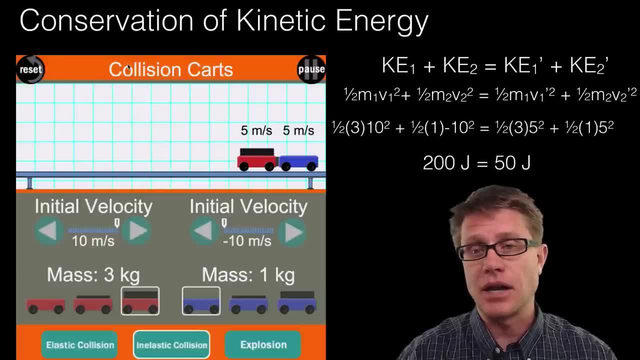 This is inelastic. Okay, Okay, This is a non-inelastic collision. So if we plug in the elastic collision, In other words, we have lost some of that kinetic energy. But you might be thinking to yourself: where did it go? Well, think about a car accident, when two 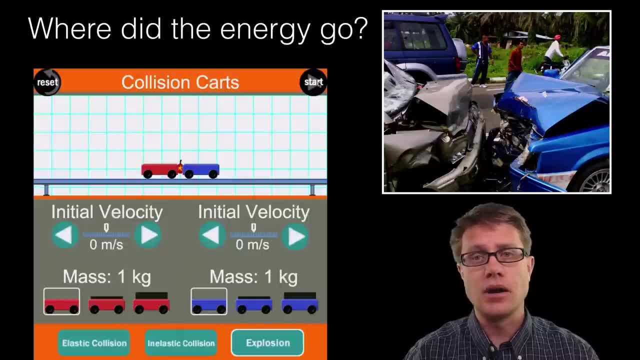 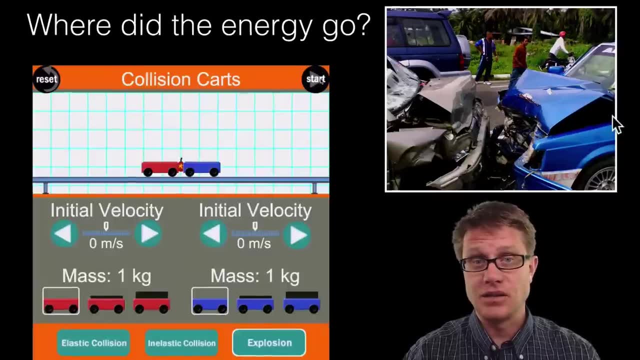 cars run into each other. They had kinetic energy before. Where did it go? It became the internal energy after that collision And we can even have a super elastic collision. So if we have an explosive device in the middle, it is all internal energy. So what is the? 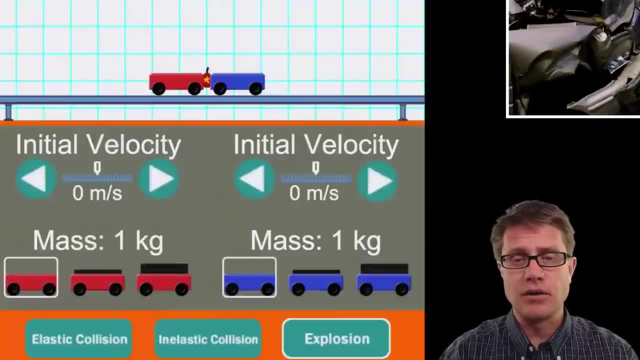 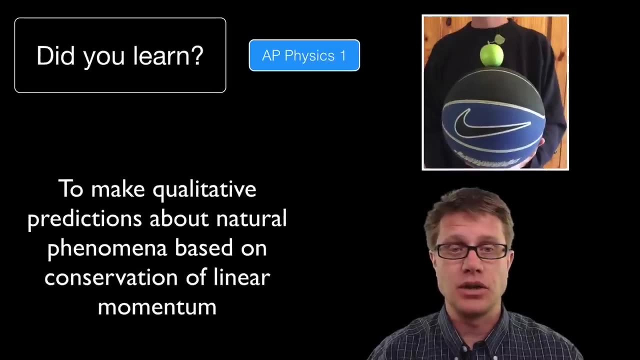 momentum. at this point There is no momentum. There is no movement. But if I were to let that explosive go, what is going to happen? We are going to convert all of that internal energy to kinetic energy in an explosion like that. So did you learn to make qualitative